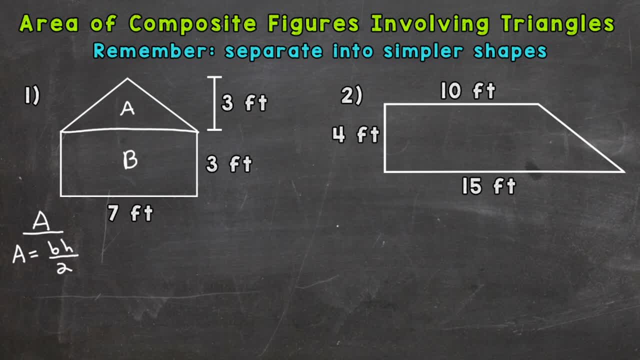 divided by 2.. Now you may use 1 half times base times height for the area of the triangle. That will give you the same answer. Dividing by 2 is the same as multiplying by a half, So let's plug in. Area equals. the base of A right here is 7 feet times the height, 3 feet. 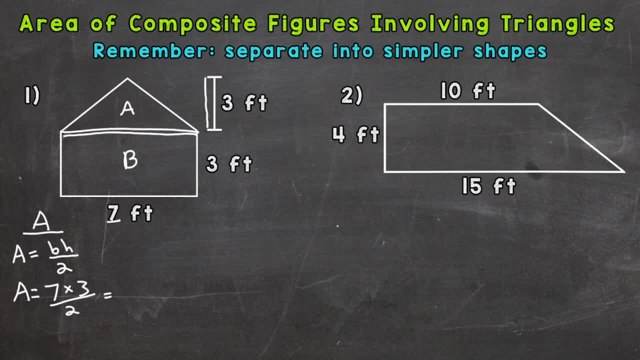 And divide by 2.. So that gives us 21 divided by 2.. So area equals 10 and a half square feet. So now we need to do B, So area of a rectangle length times width. Let's plug in: Our length is 7 feet. 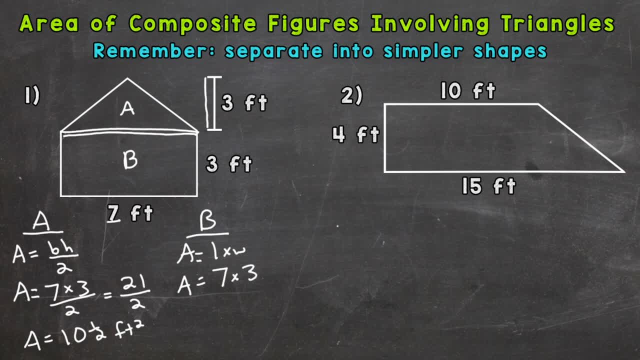 times width. Now if you did 3 times 7, that would give you the same answer, So don't get caught up on the length and width. there, Area equals 21 square feet. So now that we have the area of A and B, 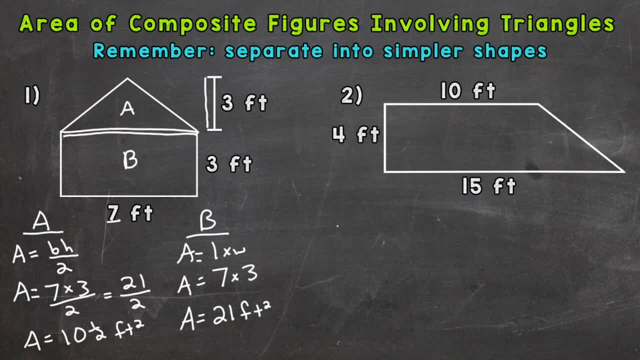 we need to add those together for the total area of the composite figure. So I'm going to come up here: Area is going to equal that 10 and a half square feet Plus the 21 square feet. So let's add those together. 10 and a half plus 21 is going to give us 31 and a half square feet. 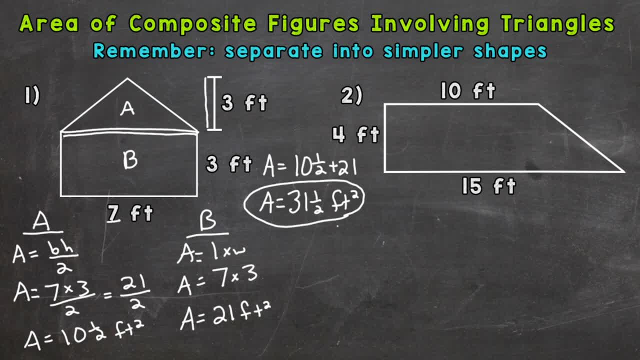 So that's the total area for number 1.. So let's move to number 2. here, Again, we need to separate into simpler shapes. So let's cut this shape right here. That way we have a triangle and a rectangle. We'll call the rectangle A. 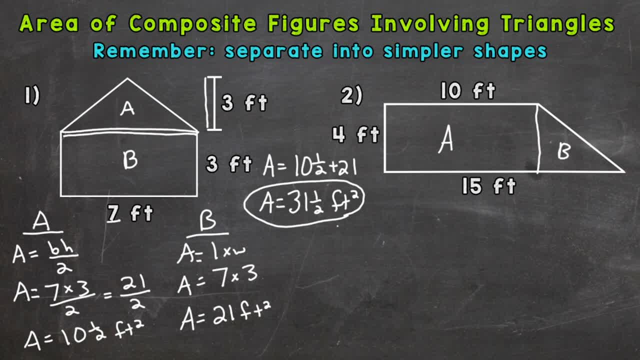 And the triangle B Doesn't really matter which one you name, A or B, or what you name them, As long as you're organized and it will all work out in the end to give you the same answer. So let's find the area of A first. 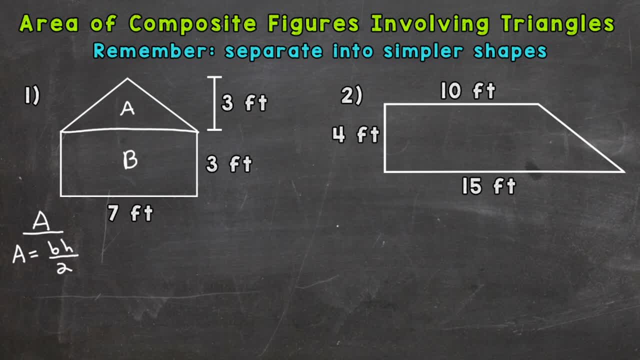 divided by 2.. Now you may use 1 half times base times height for the area of the triangle. That will give you the same answer. Dividing by 2 is the same as multiplying by a half, So let's plug in. Area equals. the base of A right here is 7 feet times the height, 3 feet. 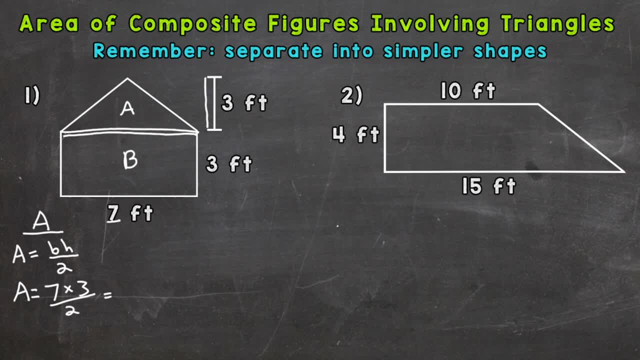 And divide by 2.. So that gives us 21 divided by 2.. So area equals 10 and a half square feet. So now we need to do B, So area of a rectangle length times width. Let's plug in: Our length is 7 feet times width. 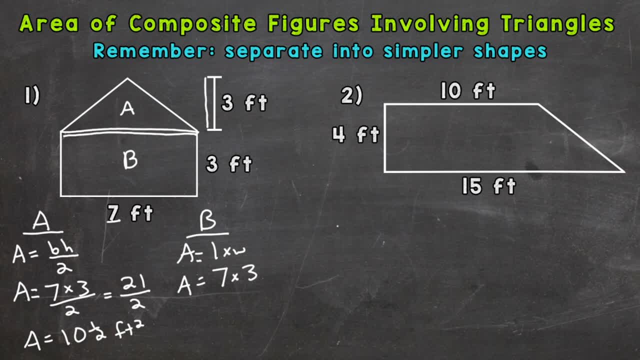 of three feet. Now if you did three times seven, that would give you the same answer, So don't get caught up on the length and width. there, Area equals 21 square feet. So now that we have the area of A and B, we need to add those together for the total area of the composite figure. 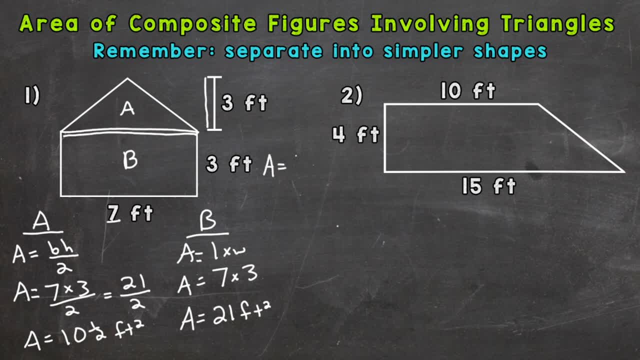 So I'm going to come up here. Area is going to equal that 10 and a half square feet plus the 21 square feet, So let's add those together. 10 and a half plus 21 is going to give us 31 and a half square feet. So that's the total area for number one. So let's move to number two. 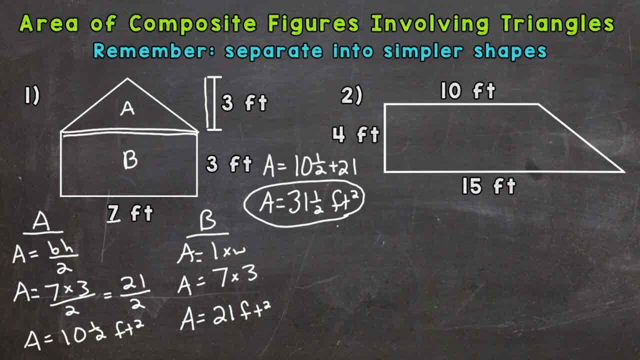 here Again, we need to separate into simpler shapes. So let's cut this shape Right here. That way we have a triangle and a rectangle. We'll call the rectangle A and the triangle B. It doesn't really matter which one you name, A or B or what you name them, as long. 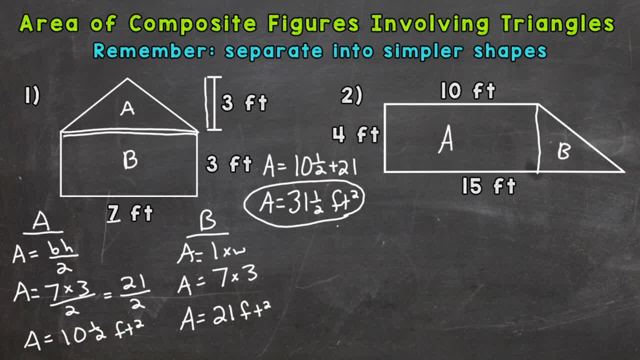 as you're organized and it will all work out in the end to give you the same answer. So let's find the area of A first. So formula for rectangle length times width. So let's plug in Length I'm going to use. Don't use the 15 feet, The 15 feet goes all the way.